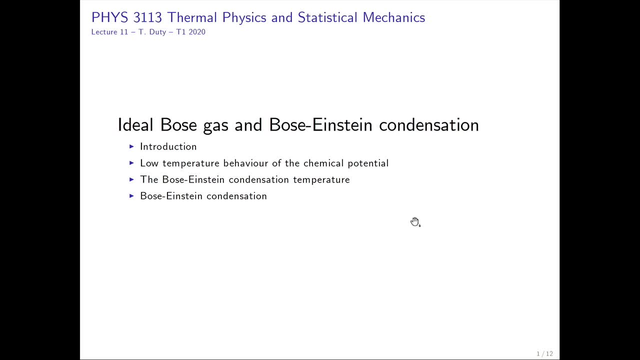 and then we'll discuss a bit more about some of its properties. So of course we have a collection of bosons or an ideal Bose gas, that is, a collection of non-interacting bosons. The properties are really quite different than those of the ideal Fermi gas and of. 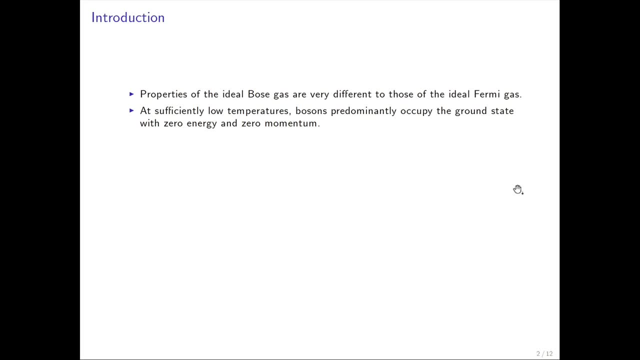 course that's because of the statistics and we'll see that, sufficiently low temperatures, bosons predominantly occupy the ground state, the ground state at zero energy and zero momentum. So we'll see that below a critical temperature, which we call the Bose-Einstein condensation, 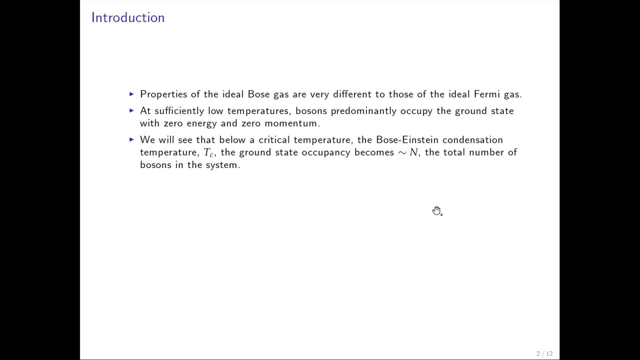 temperature, TC. the ground state occupancy becomes of order of N. the total number of bosons in the system, And in this range the de Broglie wavelength, or the so-called thermal de Broglie wavelength, becomes macroscopically large Around TC. it's such that the bosons 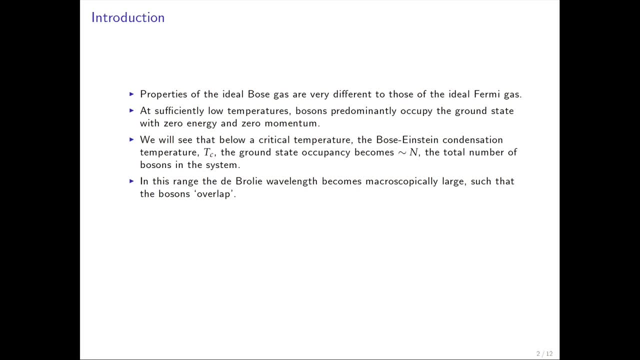 start to overlap each other and as we go to very, very low temperatures, then this wavelength becomes of order, of the size of the container that you have the bosons in, like, for example, particles in a box. And so, and it's very interesting, this phenomenon of a Bose-Einstein condensation, because the 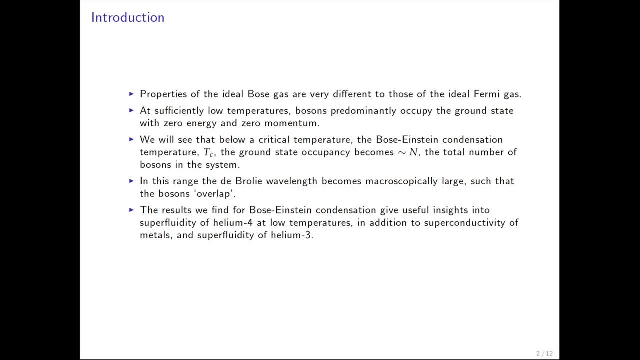 results we'll find here give a lot of insights into other types of condensation, in particular the superfluidity of helium-4, and then superconductivity of metals and superfluidity of helium-3. And these latter two types of superconductivity and superfluidity of helium-3 actually involve 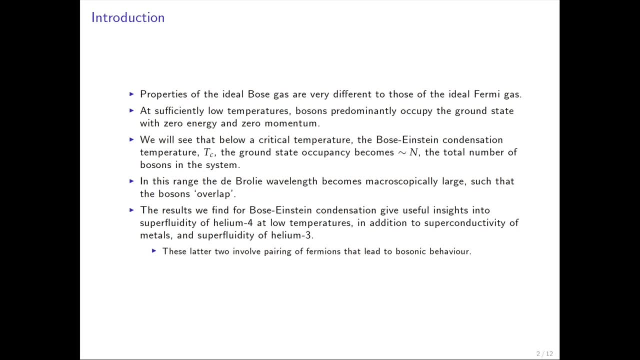 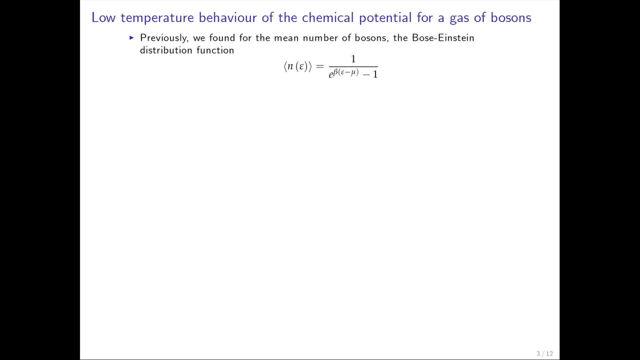 pairing of fermions that lead to bosonic behavior. We're not going to discuss that pairing in this course, but we'll just talk about non-interacting bosons and Bose-Einstein condensation, which gives a nice analogy and insights into these other systems, which are actually much more complicated. 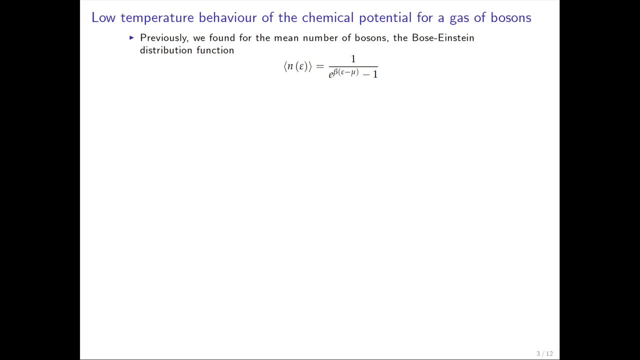 Okay, so previously we derived this Bose-Einstein distribution function, which is the mean number of bosons in some state of energy epsilon, And it has this form: 1 over e to the beta. beta here is 1 over kB T. 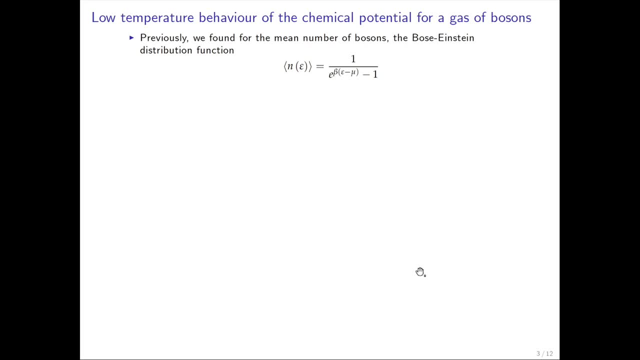 E to the beta times. epsilon minus mu. mu is the chemical potential and we have the crucial difference from fermions with a minus 1 here And we'll see that this chemical potential plays an important role in the temperature dependence of the ideal Bose gas. so we'll have to spend some time with this. 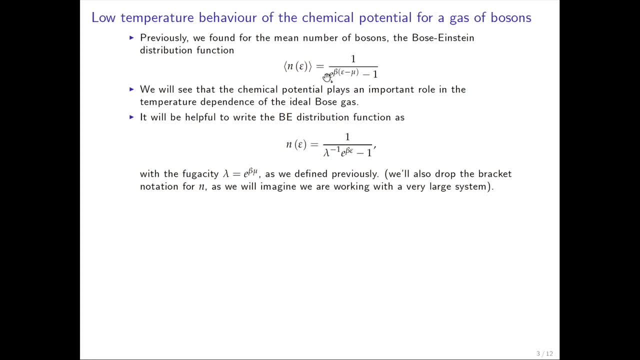 So let's just write this as we did before. We'll factor out this: e to the minus beta mu, which is inverse lambda. this fugacity, so lambda, is e to the beta mu. Let's just write it this way. And for now I'll also drop this bracket notation, which means mean value, because we're going. 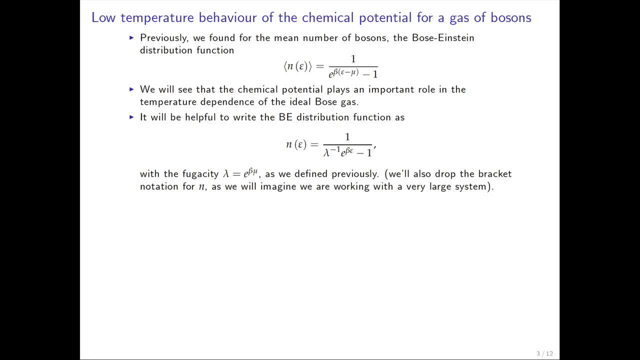 to be working. imagine we're going to be working with a very large system and we'll just ignore the fluctuations around that and take this as the number in the state. We'll be fine to do that for a large number of particles, as we've shown previously. 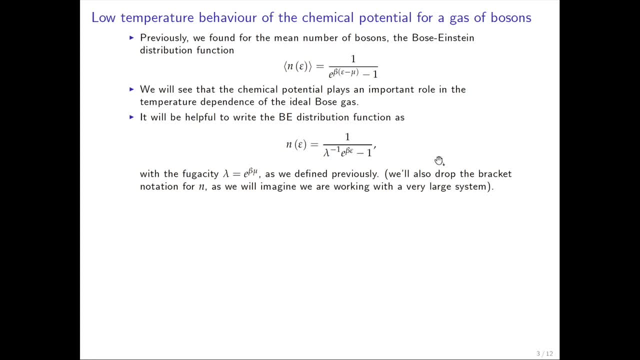 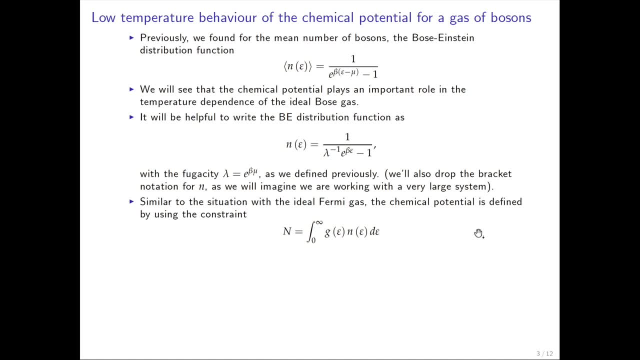 That is, we have a system coupled to a heat bath and also a system with which it can exchange particles, And the way we do that is we define. eventually, we define the chemical potential in order to fix the mean total number of particles, which we'll call just e, to the beta mu. 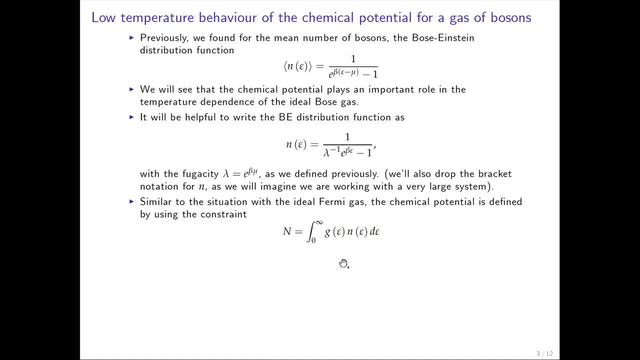 And that's just n here, capital N. And remember, we did this for the Fermi gas as well, in particular. t equals zero And we get that by integrating over the density of states times this occupancy or this Bose-Einstein distribution function. 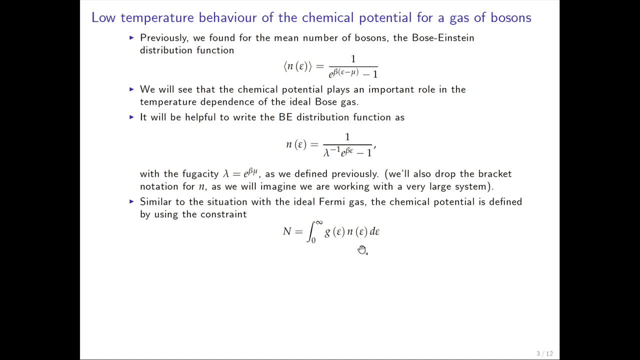 We. of course, this formula is valid for Fermions or bosons, but we'll use this function here for bosons Now, at low temperatures. as you can, by looking at this occupancy, you could see, this is that the number in the state of thermonuclear temperature is just n, and that's the probability of that. 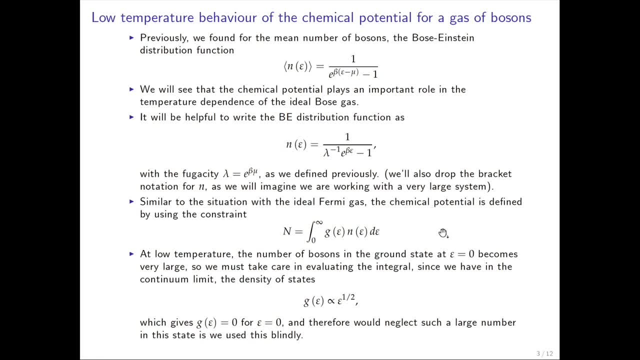 form定ing over conditions. Now let's say that this is, let's say, 1.1 times this or 0.2 times 1.1 times k, because there's no. is that the number of bosons in the ground state? 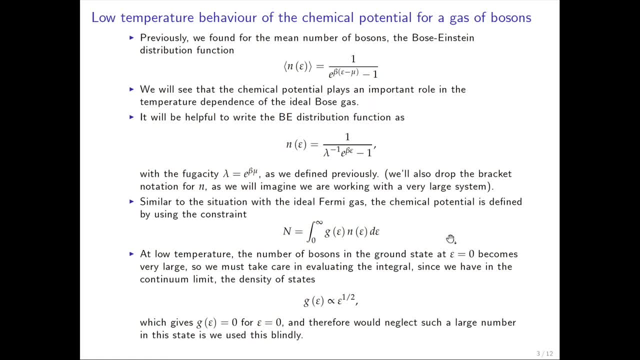 if we set epsilon equals zero here, this could become very, very large, Because you know. so we have to take, we have to be a little bit careful when we evaluate this integral, And the reason is is that, if remember, 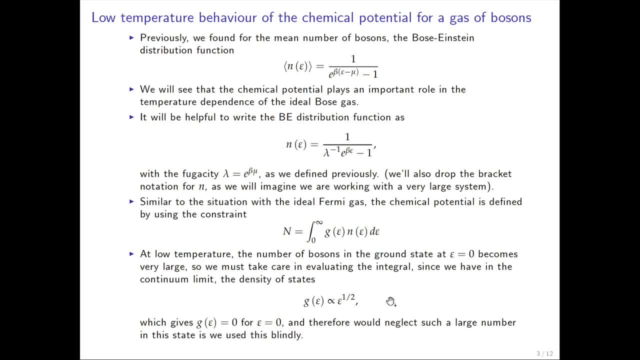 we use the 3D particle in the box states and we have this density of states that went like the square root of the energy, And of course you can see that this density of states G is zero when epsilon equals zero. So that means in this integral, 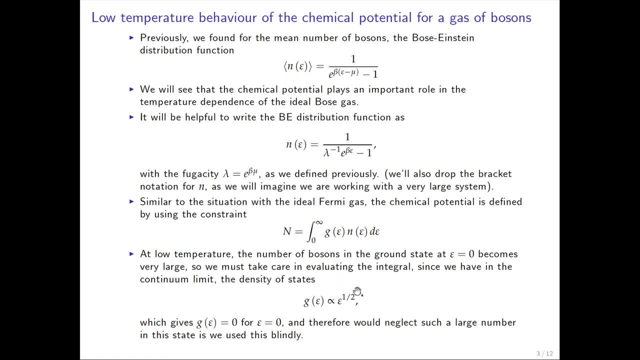 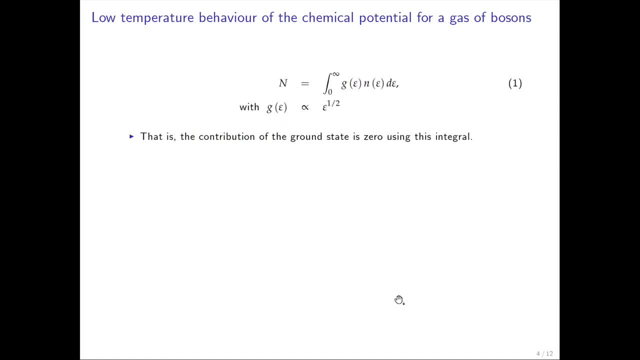 the states at zero energy, you know, are neglected. if we just use this blindly, Now, usually that's not a problem, right, Let's see. So let's just write that again. So we have this equation And, of course, if this density of states, 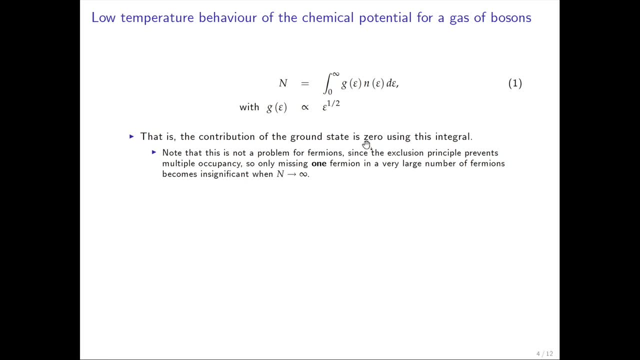 goes like energy to the one half, then it's not going to get. you know, we're not going to get any contribution from the states that sit exactly at zero, And usually that's not a problem for fermions because of the exclusion principle means. 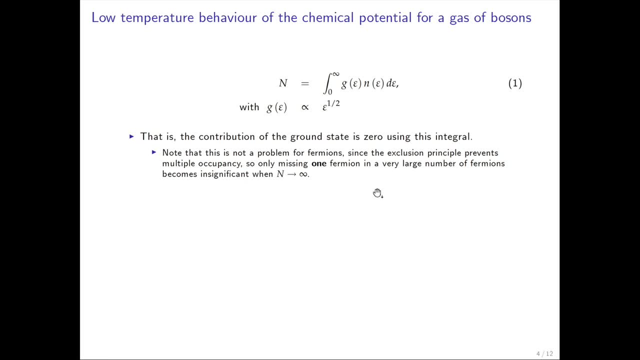 you know, prevents multiple occupancy. So you know, missing one fermion down there when we go to a very, very large number is not really going to affect anything. It's going to be quite insignificant. But that's not the case with bosons. 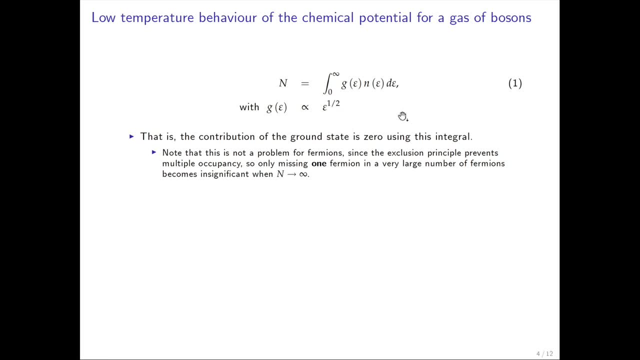 because we could get a whole lot of particles down there at zero energy. And so you know, you can imagine that you leave out the contribution there, Right, Because we've. you know we've gone from a sum to an integral. essentially. 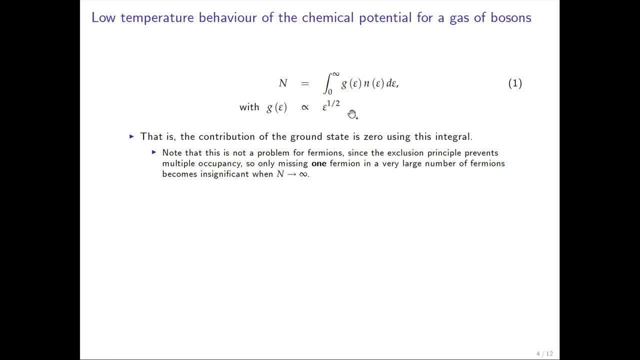 to get this density of states. Imagine we're counting a lot of states that are close together, So it's kind of an artifact of this. We just have to be a little bit careful with bosons And as we'll see what we need to do, 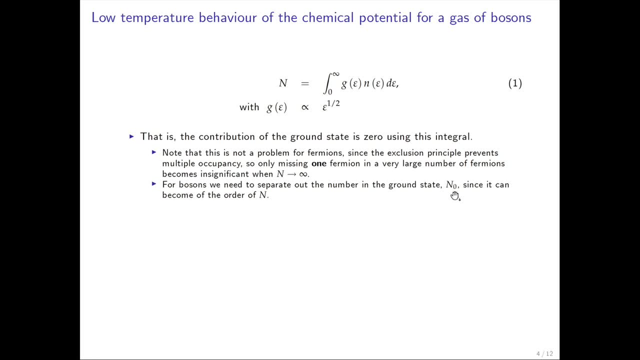 is separate out the number in the ground state that we'll call N0 here, because it can become really large in the order of the number of particles Now. so we have to kind of think about the chemical potential too, because it's really easy to see. 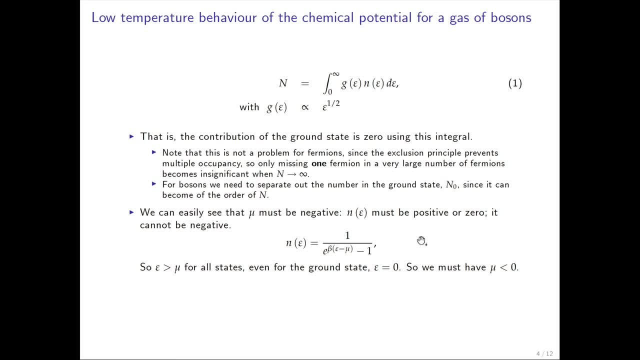 that the chemical potential mu has to be negative for bosons. We mentioned this in an earlier lecture but let's just go through that again. So you know the number in state epsilon must be. you know it's got to be positive or zero. 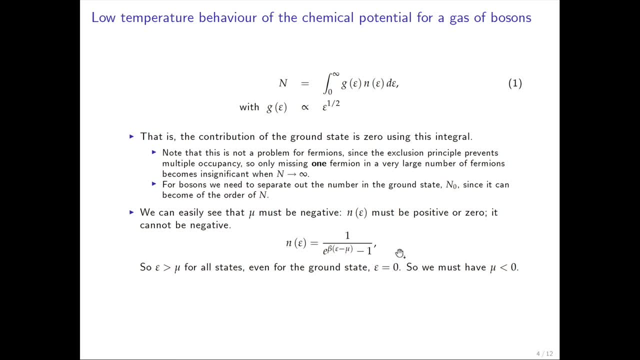 It can't be negative, of course. And so there's the boson distribution of function. And so, in order for this to be positive or zero positive, this epsilon has to be bigger than mu, right, Epsilon has to be bigger than mu. 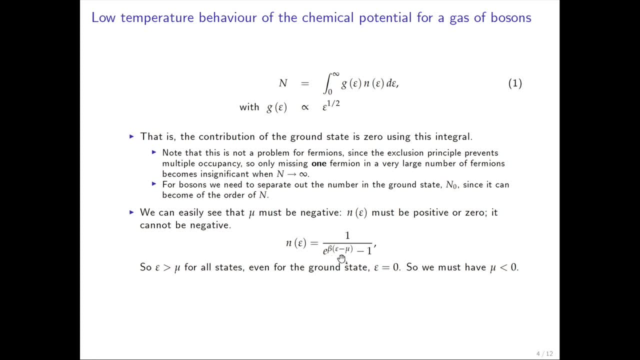 so this is positive here, I mean because? if so, let me just explain it. If this quantity were negative, right. if epsilon were less than mu, this quantity would be negative and this factor would be less than one right. And that can't happen. 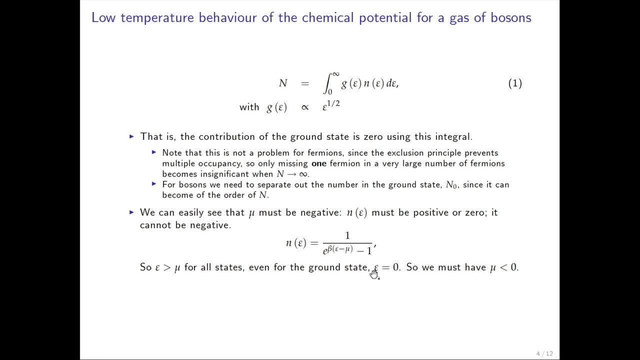 Because then that would make the denominator negative. So you know, this has to be true even when epsilon equals zero at the ground state. And if epsilon equals zero and mu has to be less than that, mu has to be zero even for the ground state. 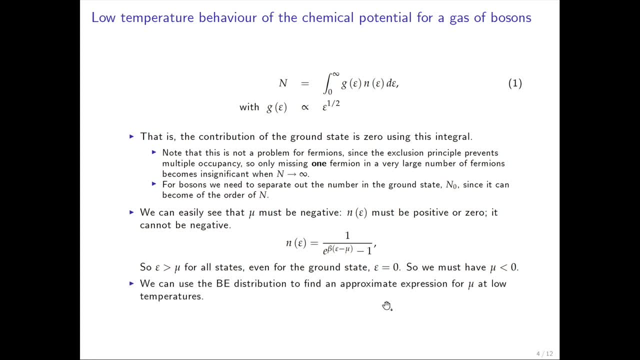 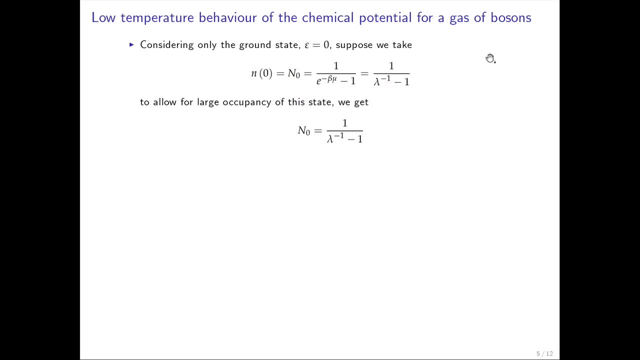 So for right. So we'll use this Bose-Einstein distribution to find an approximate expression for mu at low temperatures. Let's do this first. So so we have, for the ground state, at epsilon equals zero, the occupancy. we're going to call it big N zero. 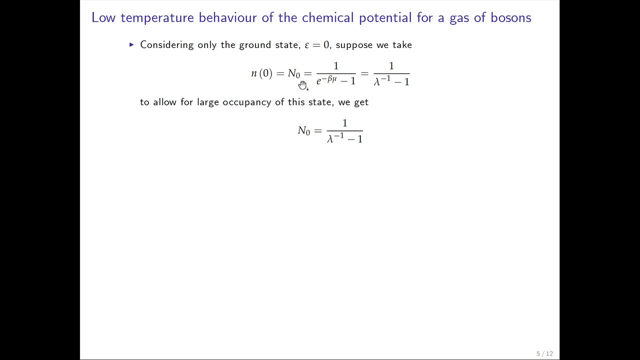 because we're going to imagine that'll remind us that that N we're going to be interested in at low temperature, when this N is big, So let's write big N, zero, And so at epsilon equals zero, of course, we just have this expression. 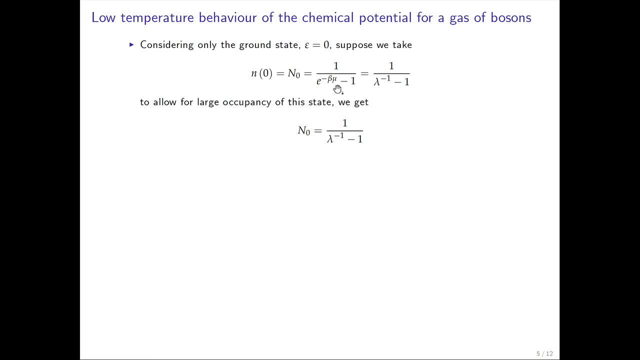 where we set epsilon equal to zero and, given our definition of the fugacity, we just have this right. And and if we solve this for the inverse fugacity, which, let me remind you again what that is, it's the fugacity is e to the beta mu. 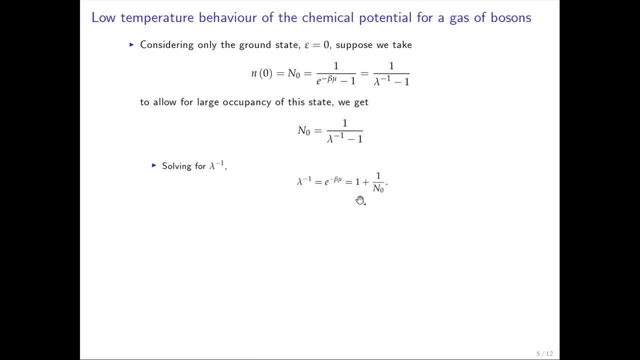 So one over the fugacity e to the minus beta mu. We just solve this in terms of that and we get one plus one over N zero And and we see, if we want N zero to be large, that means this term gets really really close to one. 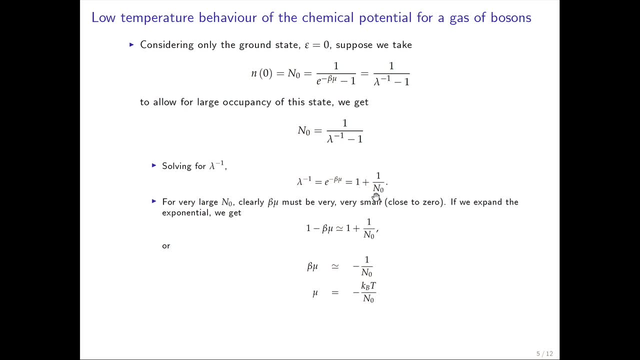 This is small. It's getting very, very close to one, And if we want this to get very close to one, then remember mu is negative. So beta mu must be be small, And and and because mu is negative, 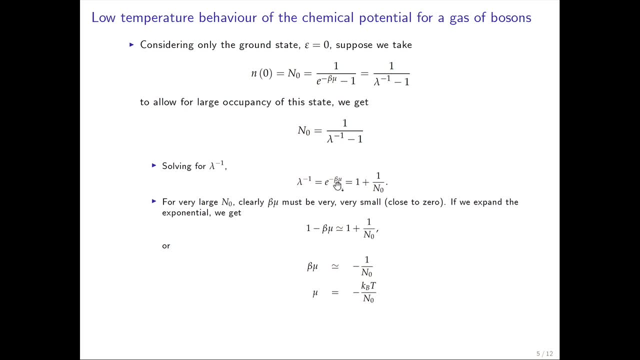 this is needs to be a small positive number, Because if it's a large positive number, this is going to be huge, And so we need this term to be near one, just just slightly above one, And that means this beta mu has to be again very. 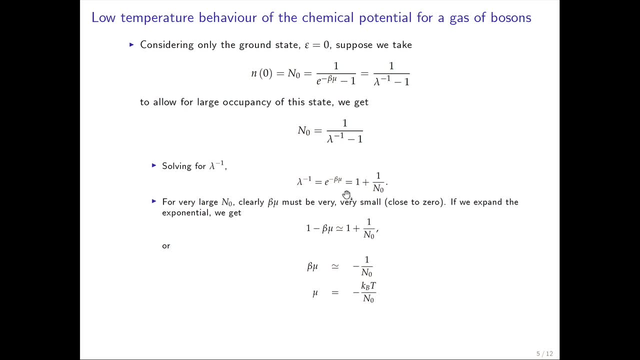 very small and close to zero. So if we expand the exponential here, so that is e to the. so. so if beta mu is really really small, then I can expand the exponential and I get one minus beta mu And then I can. and so for beta mu small, I have. 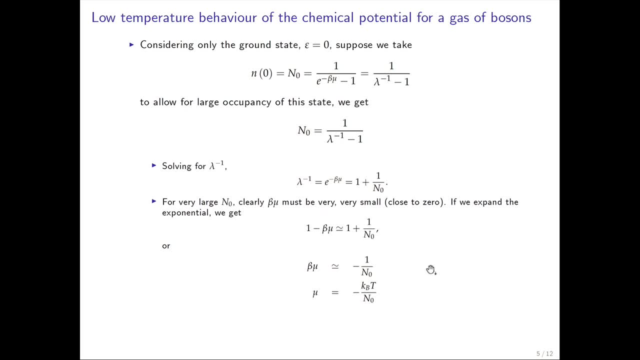 I just set one minus beta mu equal to this side, And so you can solve this, you see, And what you find is that, well, we have, we write it now in terms of kbt, right, Beta is one over kbt. 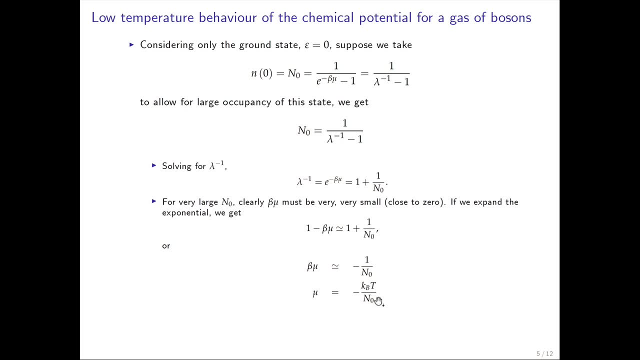 And we see that mu has to be negative And proportional to the temperature and divided by n zero. So if, as we said, if n zero is very, very large, then the mu is small and very close to zero And it kind of goes linear to zero with temperature. 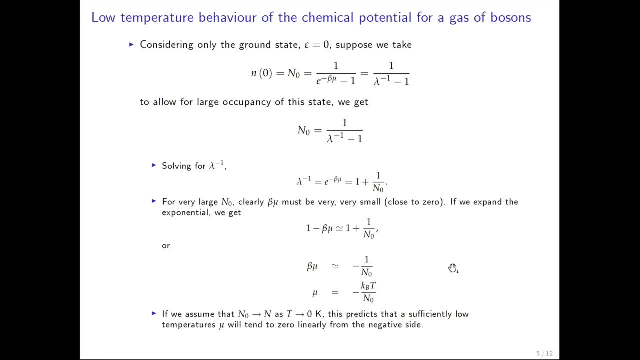 Now, as we'll see that you know, we imagine that, as as we get to very, very zero temperature, we can see from the Bose distribution function that all the bosons are going to, you know, go to zero. So we want to be down there at zero energy. 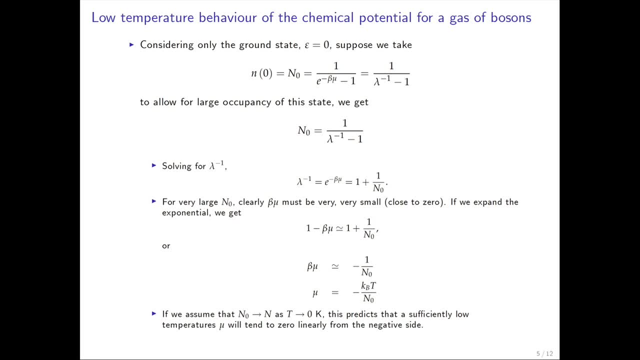 So if we we assume that n zero goes to n, the total number of particles as t goes to zero, it predicts that mu does this. That it that it goes to zero linearly. It's negative, as it has to be, as we said. 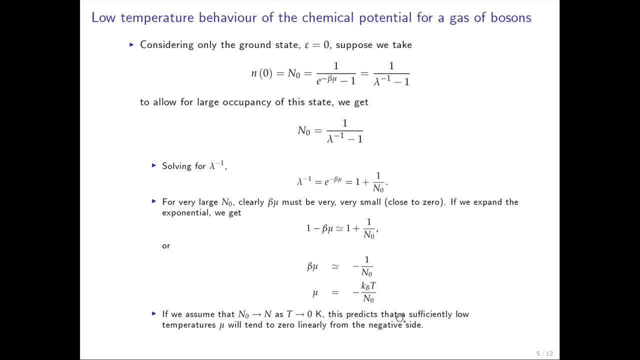 But it goes to zero linearly from from the negative side. So it goes like like temperature right. We'll see exactly how this goes later, But that's our argument, So we know. So so inclusion mu has to be negative and it gets very. 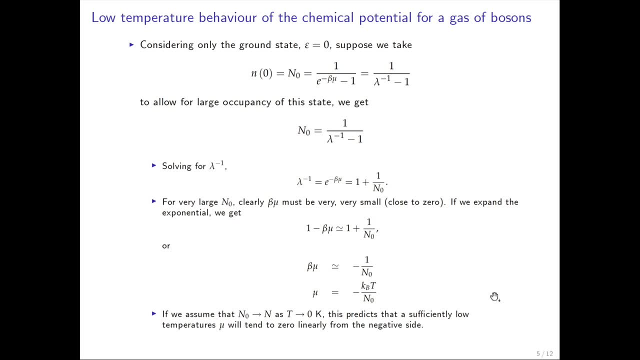 very close to zero as we go to low, low temperature. Okay, And that we got by assuming that a large number of particles were in the ground state, which we know has to be because of the Bose-Einstein distribution function. Okay, There we go. 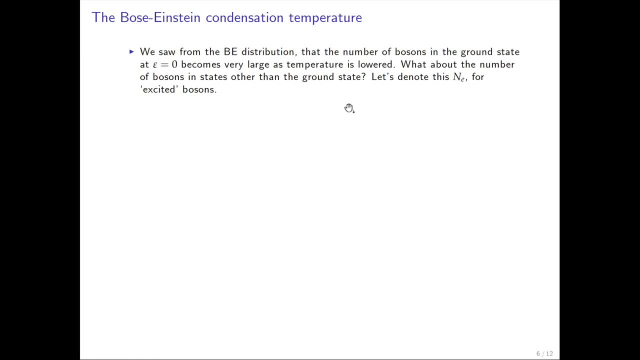 Well, so we saw then that number of bosons in the ground state, the zero energy, becomes very large as the temperature is lowered, And we worked out what that meant for the chemical potential. Well, what about the number of bosons in other states? 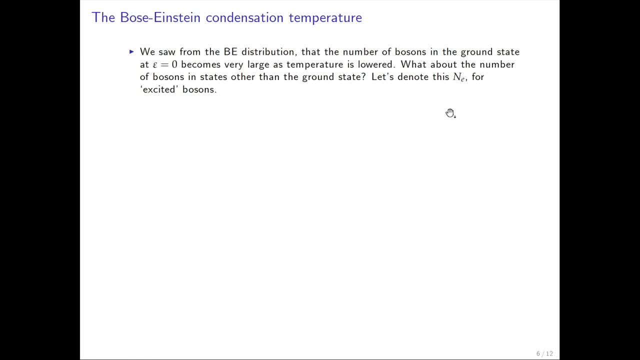 in states other than the ground state. So let let's denote this n sub e, e for excited bosons. What about the number in in the ex? that's not the number not in the ground state. Well, this, of course, will just be given by the integral. 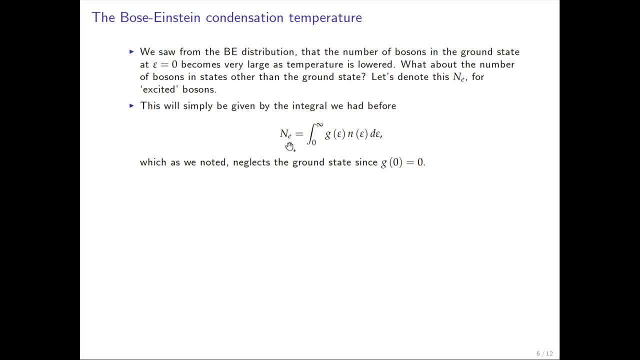 that we wrote down before. We'll just call it n sub e here, But it's, it's exactly the same. integral, Because, as we said, this neglects the, the number that are sitting down there at at zero energy. Because, because this density of states is zero, at at zero. 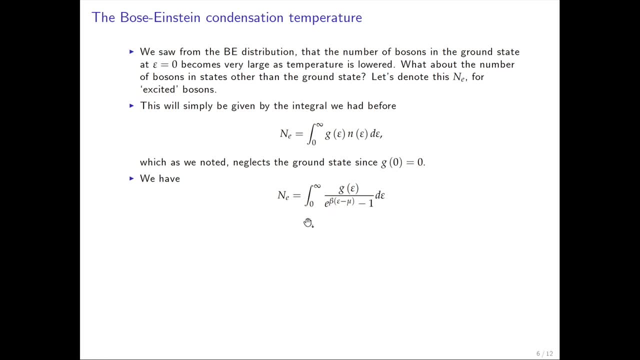 So, so, if we so, we can calculate the number in the excited state in the usual way by doing this integral. And once again, let's you know, let's assume single particle states, that is states particles in a box, states. 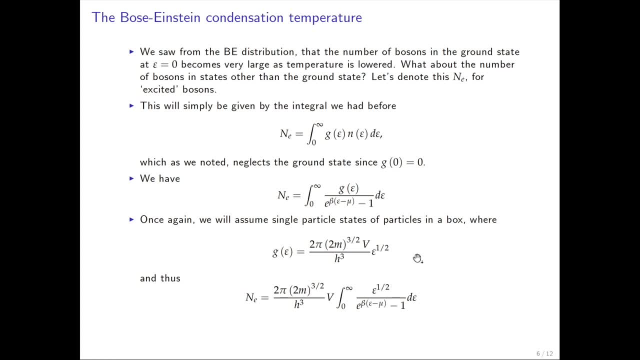 where we derived this density of states And in in in prior lectures. So so this density of states has nothing to do, of course, with whether the particles are bosons or fermion fermions. It's just the levels that you get from quant, you know. 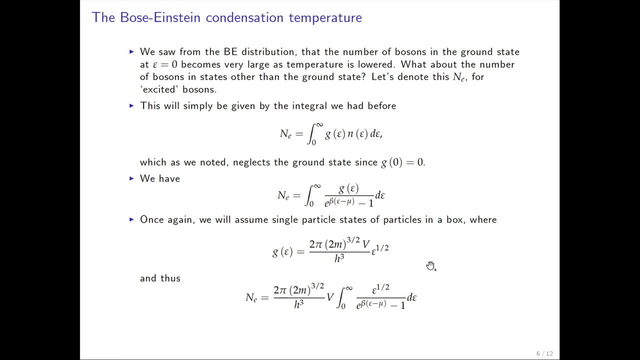 quantizing particles in a box, And so we had this expression. It goes like the square root of epsilon, and it has this pre-factor, And that's proportional to the volume, of course, And so, though, so we can do that integral. 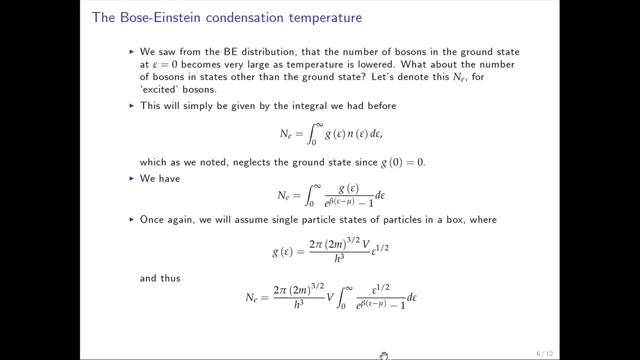 And so now we have integral, like we saw for fermions. we're going from zero to infinity here of this function, right? Well, so that's the number of particles, not in the ground state. Now, like we said, you know, 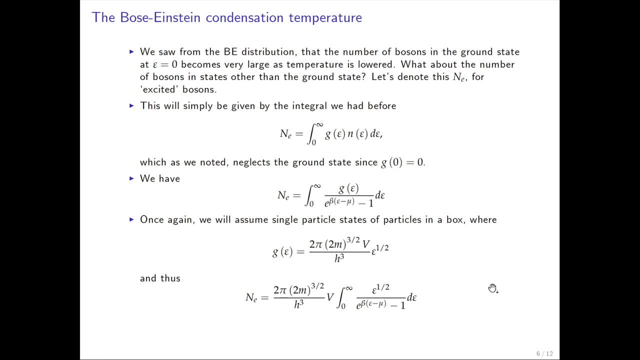 if we didn't have to worry about the particles in the ground state. we could say: you know, this is the total number of particles. So you know what if we let's do a kind of thought experiment? What if we wanted to keep all the total number of particles? 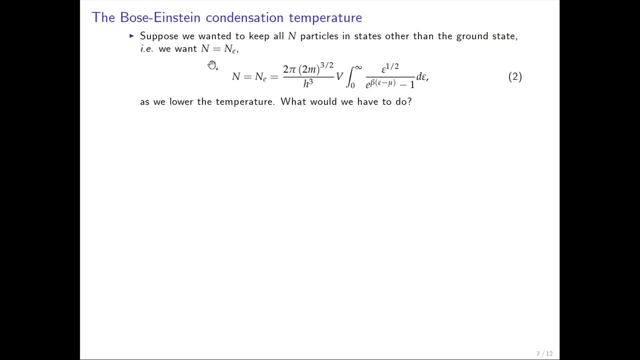 in states other than the ground state. That is, we wanted the total number of particles to be this number And remember, we can always adjust, we always find the chemical potential by this essentially constraint given by the number of particles. So let's suppose that we wanted all the number of particles up there. 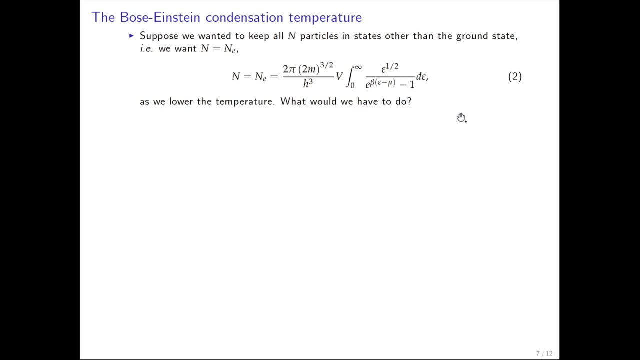 Let's look at this interval. You know, and suppose we lower the temperature. So you know we have some number of particles and we're not at low temperature, where mu, you know, is completely arbitrary, close to zero. It's some value. 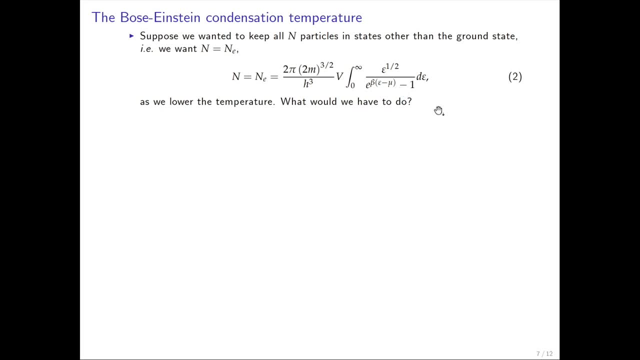 Mu is some value, you know. And suppose we then lower the temperature, And what would you have to do to keep in the same right? Well, you look at this and you say: well, as I lower the temperature, beta is getting larger, right? 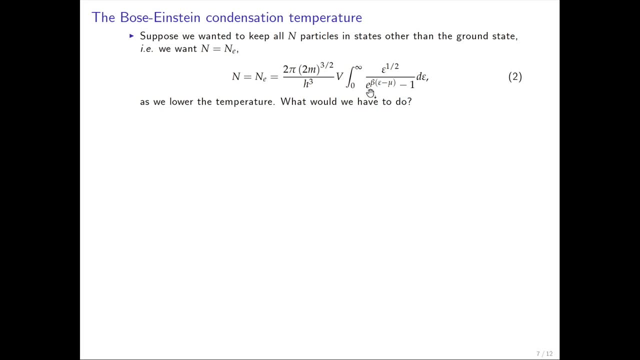 And so this factor, this factor here, is starting to get larger. And then so the denominator is getting larger, because this factor is getting larger And this thing in the interval is getting smaller, And if I want to keep in the same value I've got to change something here. 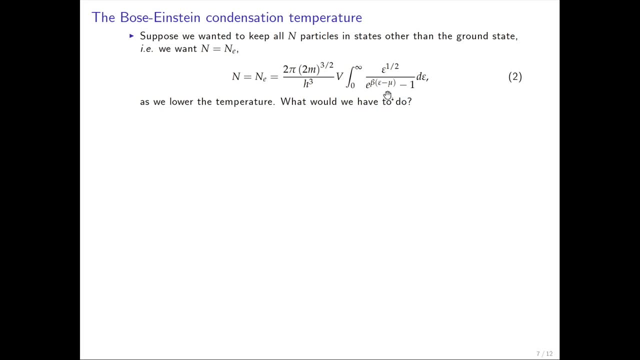 So I've got to actually change this factor to compensate for the beta thing making it smaller. And the way to do that is, of course, to adjust the chemical potential. And the way to do that is, you know, if we lower the temperature, mu remember which is negative. 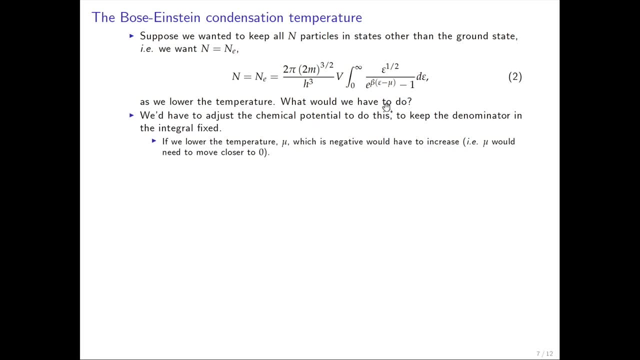 we would have to increase mu, So make it less negative, right, And so this term. so if beta is getting larger, we need to make this term smaller, which means making mu closer to zero. okay, If we wanted to keep this fixed. 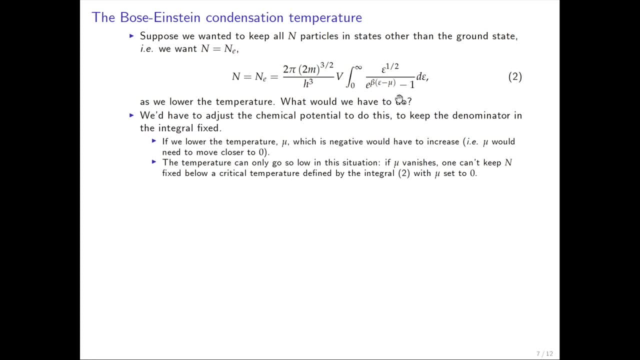 And this you know, and what you see then is that you can only, the temperature can only go so low in this situation, because we can't arbitrarily make mu well, we can't make mu positive, So if we need to make it, push it closer and closer to zero. 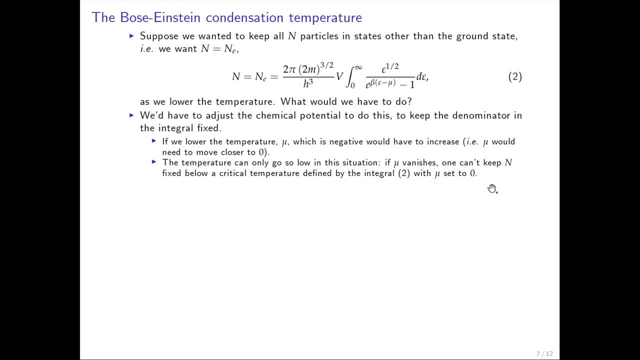 at some point. you know, we can't push it beyond zero And so if we keep lowering the temperature then we can't make this factor, we can't compensate this factor to keep n fixed right. So this actually defines a critical temperature. 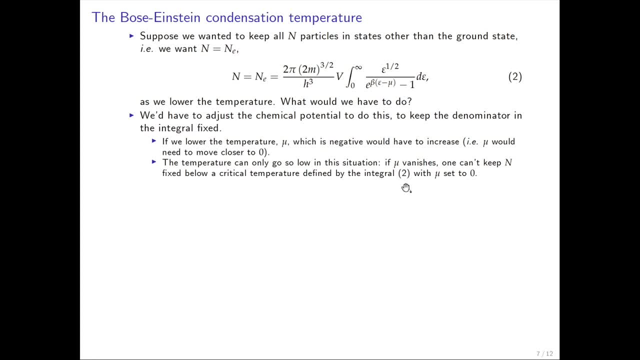 below which we can't keep n fixed, And that critical temperature can be found by doing this, of course, when we set mu equal to zero. So let's define this. So, in other words, the critical temperature is going to be defined when this by the value of this integral, with mu set to zero. 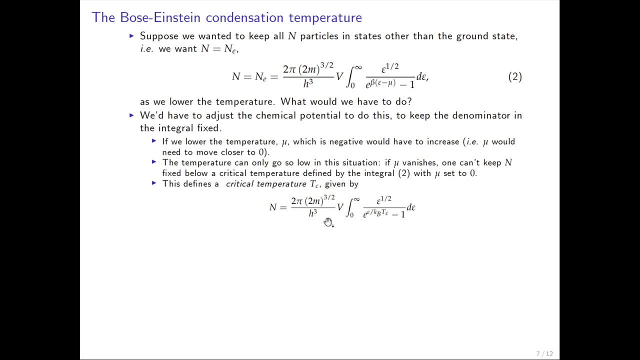 And so we can do that integral, right, We just put here the, just the constants here, And then we have this integral with mu set to zero, And I've written it instead of beta, I've just written it kbtc, because that's the critical temperature. 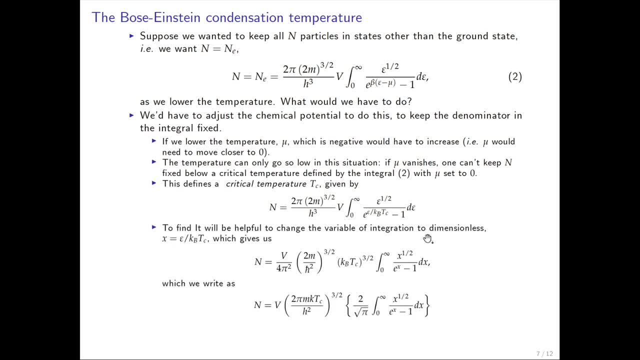 And so we could do this integral. but it's actually helpful to change our variable of integration to some dimensionless x. So we have in the exponent here, we have epsilon over kbtc, So let's call that x, Which is a dimensionless variable. 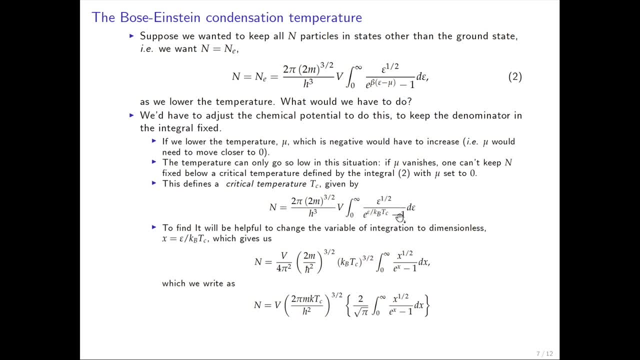 And we'll change the integration variable to this x And of course that brings out that this factor, this is proportional to epsilon one over kbtc. And of course if we change variables to x here we get essentially x to the power. one plus one half is three halves. 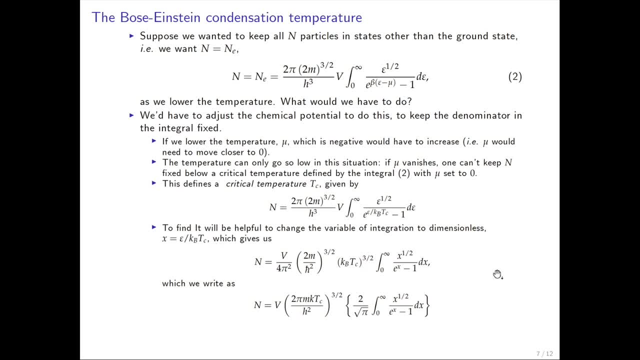 So we get this constant, of course, the three halves out here, And then we have this integral left over here, And so I'll write this integral by taking these constants and I'll take out another factor here of two over root pi. 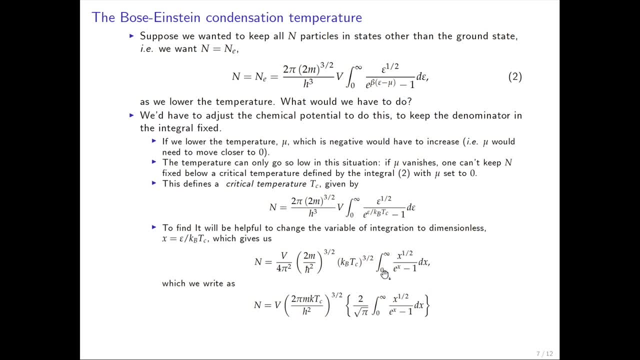 So I'll just kind of change the variable. This is a dimensionless integral and I brought it out of the side, but I'm just going to put back this two over root pi, and it'll become clear why I do that in a minute. 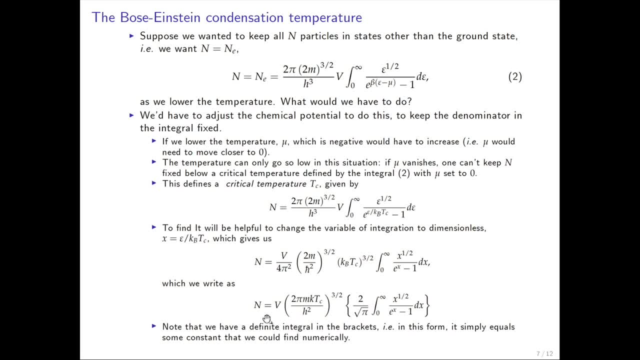 And so we have it, this form. So, basically, that's all there is really to it, because if you think about this, this integral here is a definite integral. It's an integral. it's an integral from zero to infinity of some x. 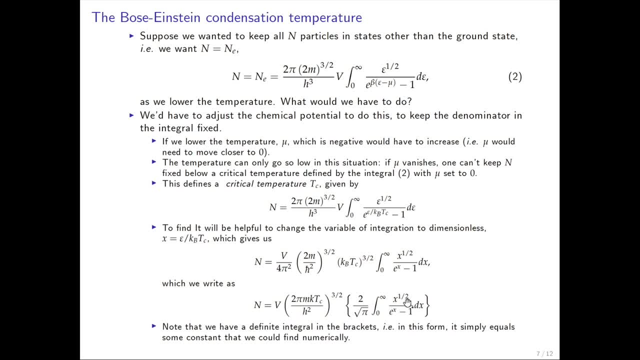 There's no other constants or anything here. So you know, this integral is just going to be some constant right And we could find- I mean, if you want to, you can find that numerically It's just so. this is just a constant, this definite integral. 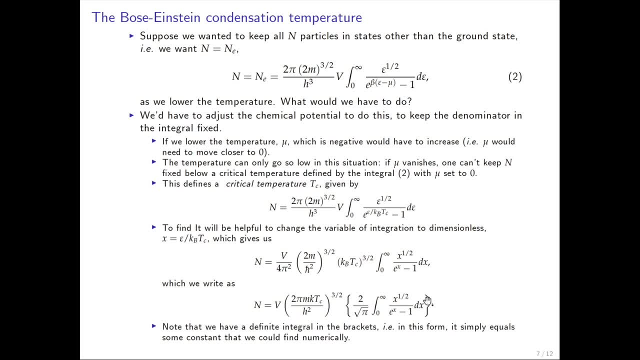 And the reason why I've written it like this is because this integral is actually recognized and has a name and we'll find that. But at this point you could just you could say, okay, that's some constant. Okay, Let me link it down a bit. 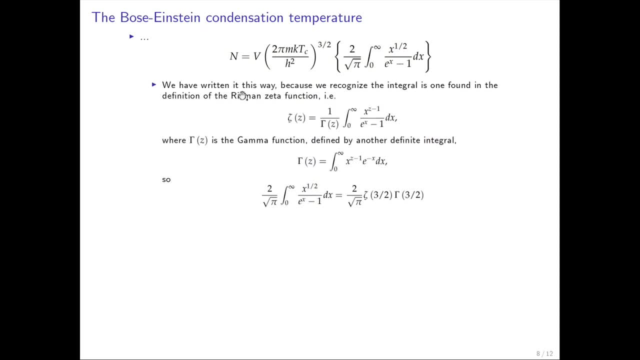 Okay, that's what we had, And so I wrote it this way, because one recognizes this integral and it's one that's found in the definition of the so-called Riemann zeta function. You may have had that in another course. 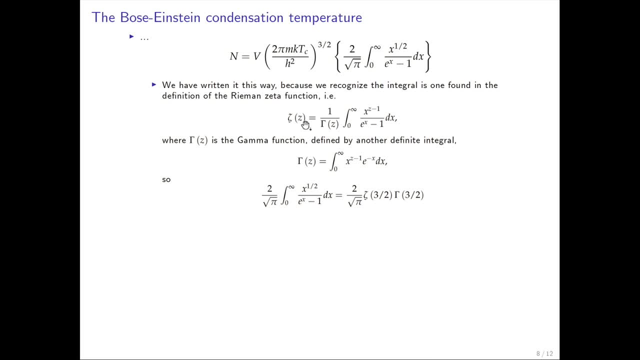 And the Riemann zeta function, the function of z. this is zeta of z. okay, it's one over this, this gamma of z, which is another definite integral, so another number times this integral right, And so you can see that our integral here. 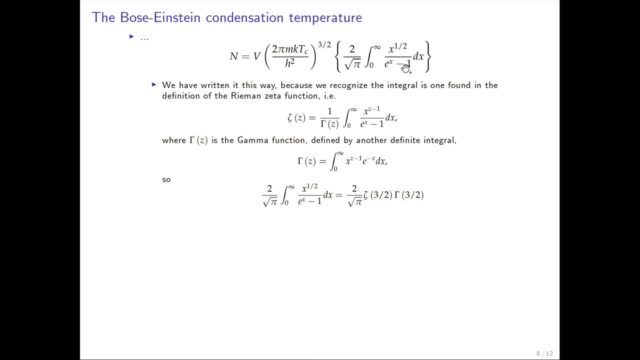 is basically z equals three halves right And so, and gamma z is defined through this integral here. but you always know it's actually a definite integral, It's just a number as well. So basically, this integral here is equal to two over square root of pi. 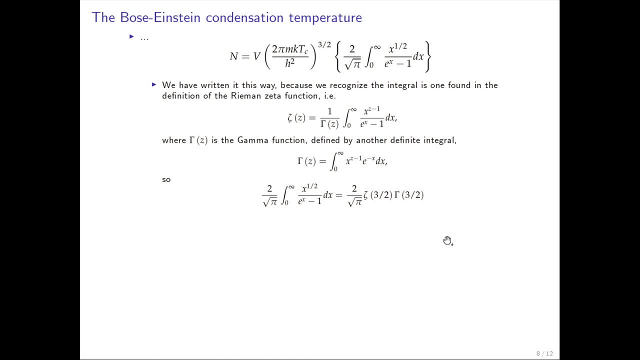 times the zeta function of three halves, times the gamma function of three halves, And the gamma function of three halves is known. it's just this. you can do this, the integral, and if you go off to a program, and it's a good enough program. 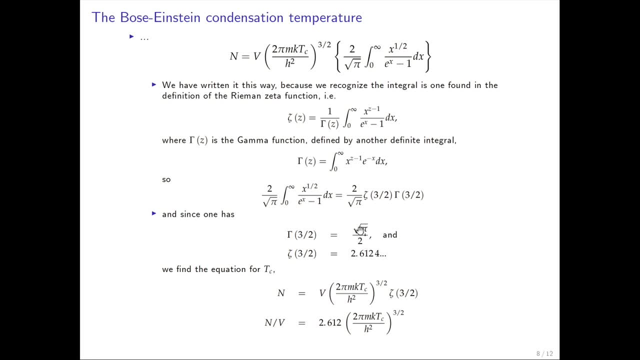 it'll find that. but it's actually square root of pi over two, which is why I pulled this factor out. And this Riemann zeta function here of three halves is just. it's a rational number. So I'll just take a few decimal places. 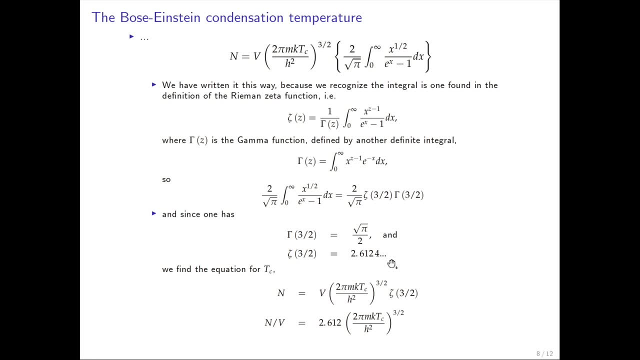 It's just this value: 2.6124 and so forth. Okay, So that's why I wrote that. So now we have this result kind of written out quite easily. This, like I said, this is just a constant. This integral becomes this constant here. 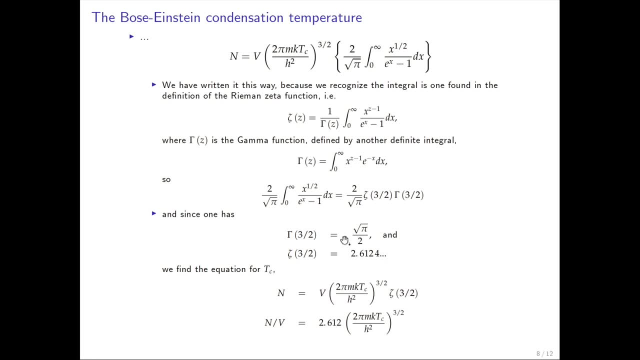 Zeta function of three halves And so- and this is just from before, So actually- and I've just moved the v over here- So basically, TC is defined now by this equation that we got. Okay, Let's write it for TC. 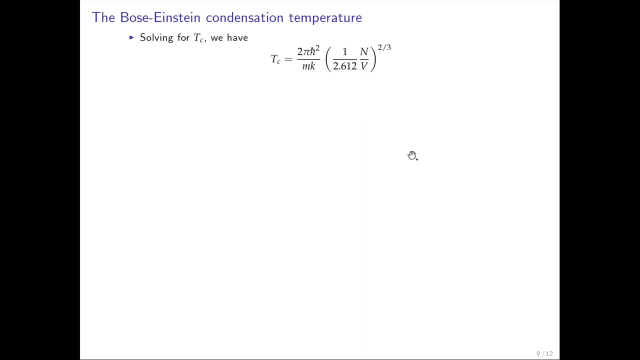 It's just that. Okay, So we found this critical temperature, you know where mu equals zero, where you know the number of particles, essentially in the excited state. we couldn't fix the number of particles in the excited state. 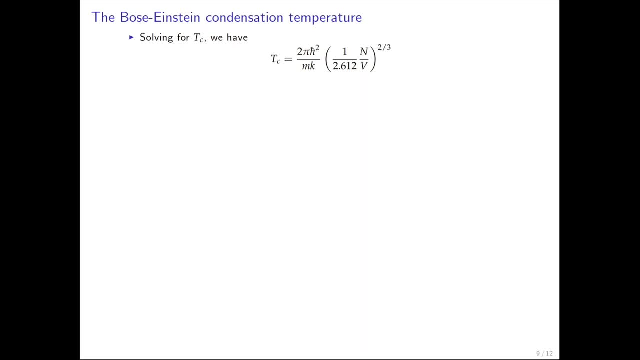 or we couldn't fix the total number of particles if we wanted to do that In all the states except for the ground state. So what does that mean? That means below this temperature we must have all the a lot of particles starting to go. 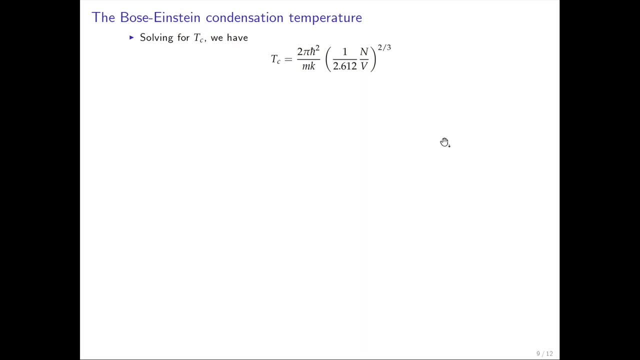 into the ground state of epsilon zero, just like we sort of argued at the beginning of this lecture. Oh, by the way, I should say you could easily go through the same integral and put a factor of S you know, out front here. 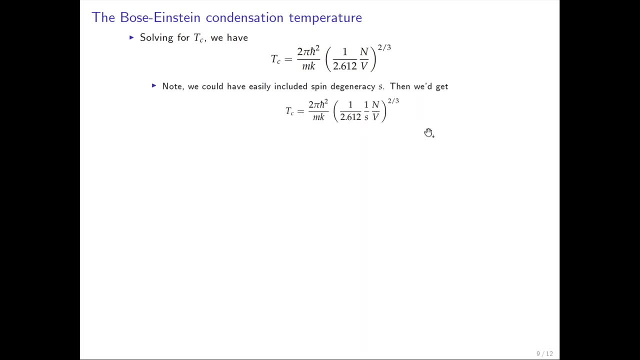 And you would just have the S downstairs as well. So, to summarize, in for T, less than some critical temperature given by this expression. we can't keep, you know, all N particles out of the ground state by adjusting the chemical potential, because you know. 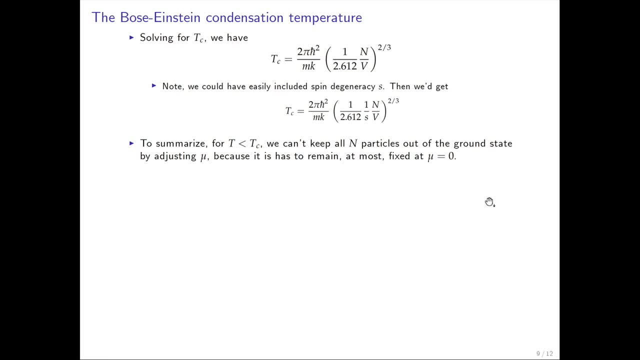 the most it can be, is fixed at zero. So that defines this critical temperature. So to make progress here we're gonna have to, you know, separate out the contributions and to see what's going on. And so we do this by writing, of course. 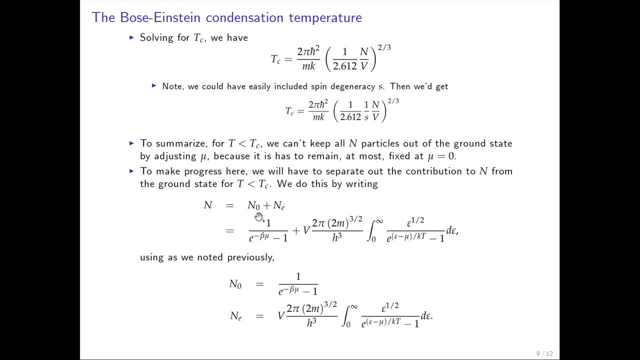 N goes in zero, So we're gonna have to do this by writing. N goes in zero plus the number in the ground state, energy zero plus the number in excited state And, as we had before, this number for epsilon equals zero, is just that term. 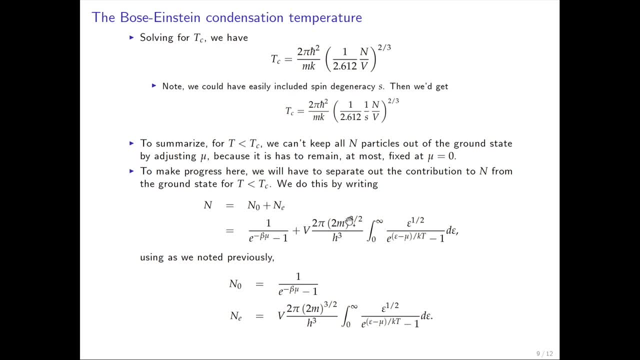 And the number excited state is just this thing we figured out before, except at some arbitrary T right, And so this is a function. This is what we get for arbitrary T below Tc. So this is a function. This is what we get for arbitrary T below Tc. 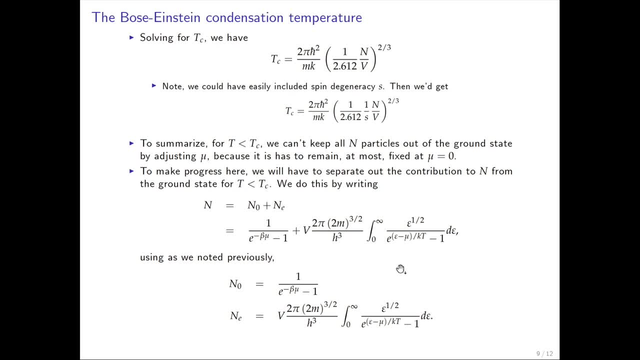 So this is what we get for arbitrary T below Tc. So this is what we get for arbitrary T below Tc. Well, I mean this. actually this expression works for arbitrary T, but we're gonna look for T below Tc. 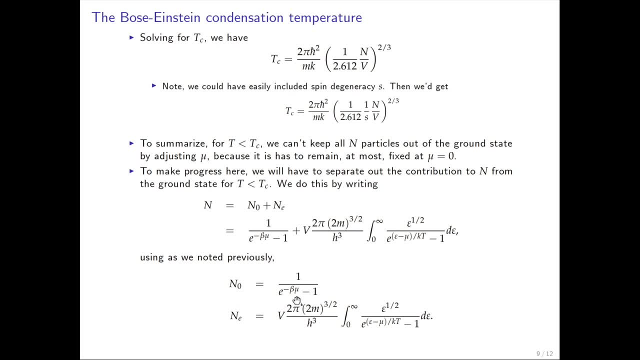 But we're gonna look for T below Tc. So, and as we found before, N zero is just, of course, this factor and the excited part is just this integral we did here with KT. I left out the B, but KBT. 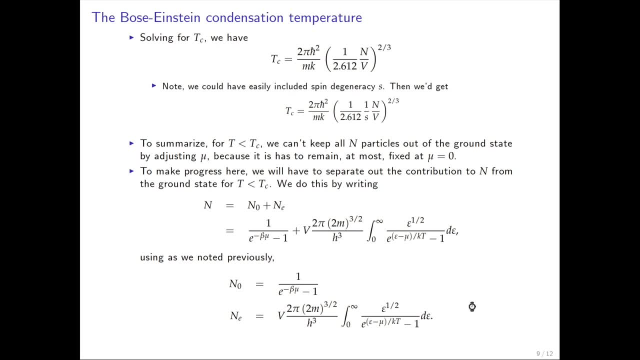 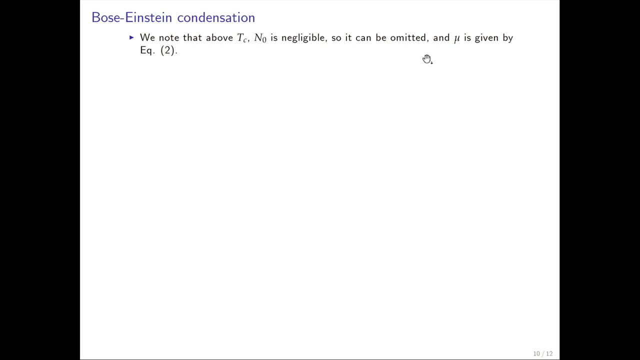 I left out the B, but KBT. Okay. And then, and we also note that, above Tc, and we also note that above Tc, we'll realize that this, we'll realize that this N zero is negligible and we can admit it. 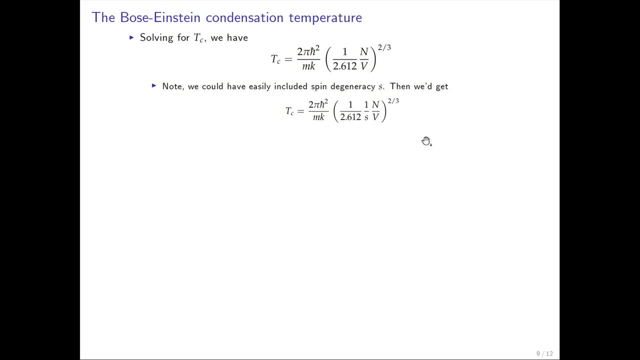 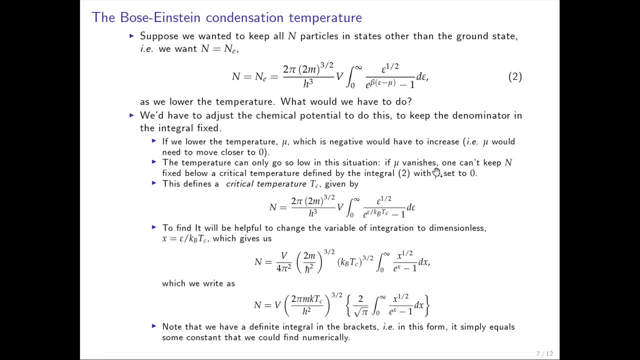 and mu is given by this equation and mu is given by this equation. We can ignore, for T, above this critical temperature. what we're saying essentially is that we can ignore the small occupancy, is that we can ignore the small occupancy of the ground state. 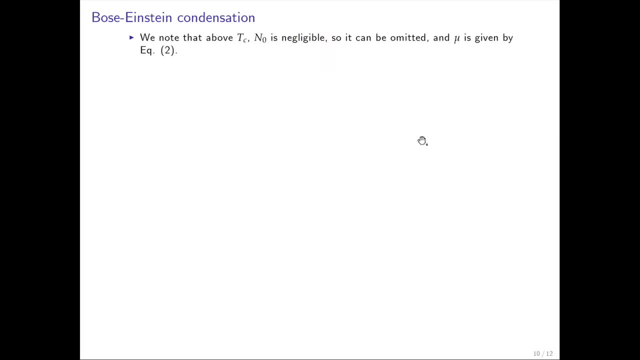 and just use this expression. and just use this expression. But below Tc this chemical potential stays really really very close to zero- And we'll see how close a bit later- but that's what our arguments or our calculations are telling us. 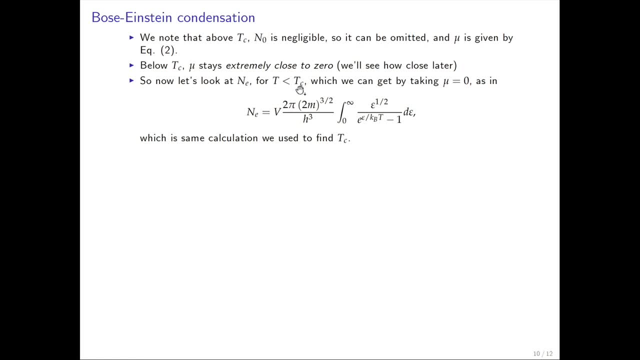 So now let's look at the number in the excited state for some T less than Tc, which again we can think by taking mu, equals zero in this expression, Because mu below Tc is extremely close to zero, is extremely close to zero. 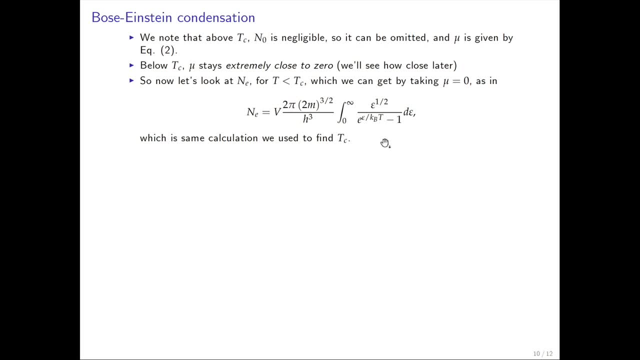 And so again we have this expression. And so again we have this expression again with now T, some arbitrary thing, and we have all these constants and it's really the same calculation we found. we used to find Tc by wanting this to be the total number of particles. 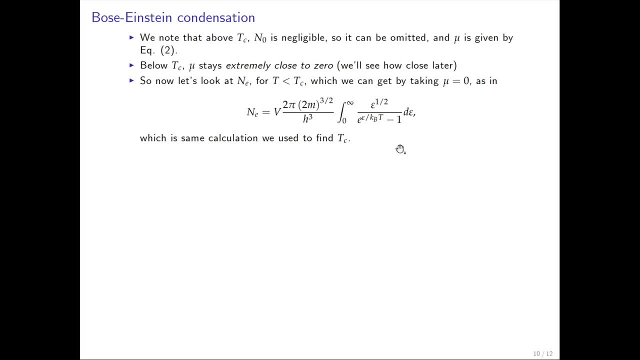 But now we're going to say it's the number in the excited state and it depends on temperature, and basically we could work this out and we would see how this- the number of excited states- depend on T and Tc, Because Tc is some combination. 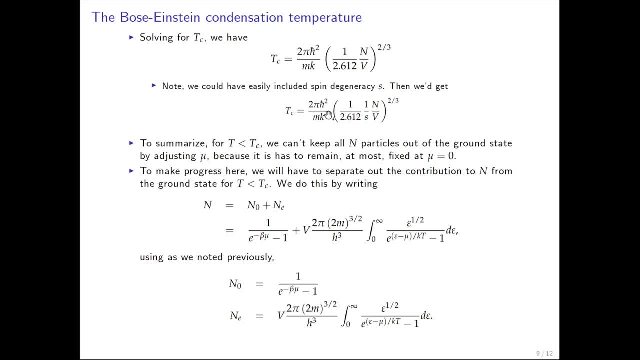 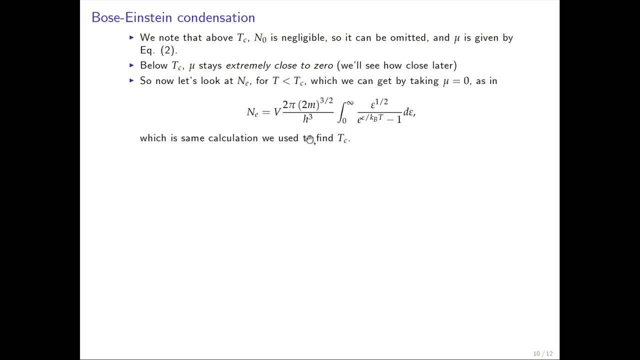 Well, if you remember what Tc is, it's this factor here, it's this factor here, And so you could completely do this integral again as it stands now, and then you would find that the expression you get has a bunch of the constants that you could find. 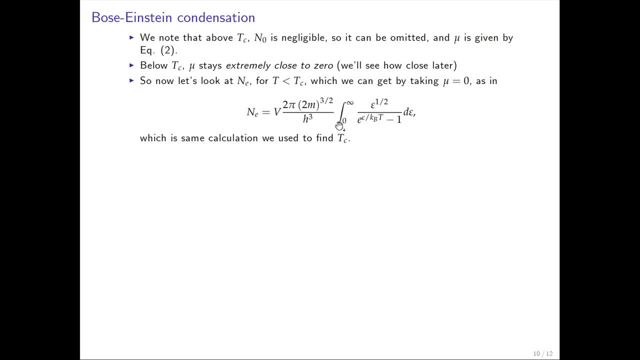 are related to Tc- the Tc found before, And you can do that if you want. but there's kind of this cute trick we can play again with this problem as well. we can write the density of states in terms of this Tc by doing this trick we used before. 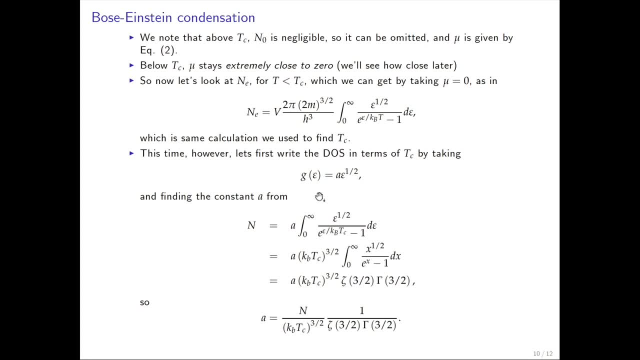 just say that well, it's some constant times, this dependence that we had, and then we go back to the equation for Tc and we can actually find what that constant is instead of in terms of all these factors here. basically, and lo and behold, it's very easy, it's the same integral we've done before. 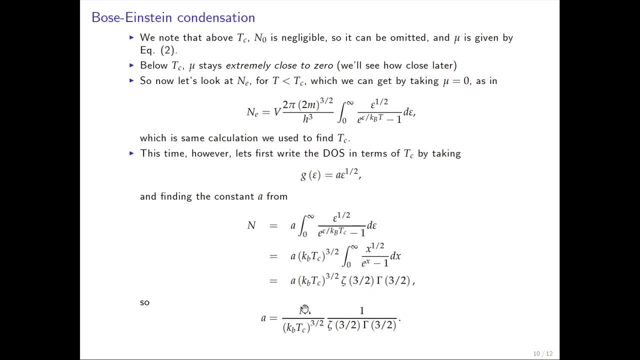 and so forth, and so you can find that A expressed as Tc instead of volume and mass and H and all that stuff is something like it's just N over KB, Tc to 3, halves, of course, times these constants again. so in that form it's very easy. 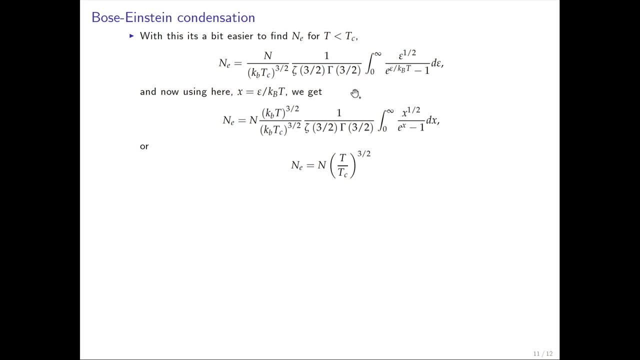 to find Tc. we just do this integral and of course that makes the whole situation very simple. we have this thing that we recognize this integral again and we change variables and this gets cancelled. this integral, once we change variables, this cancels out that. so this integral equals that in the denominator. 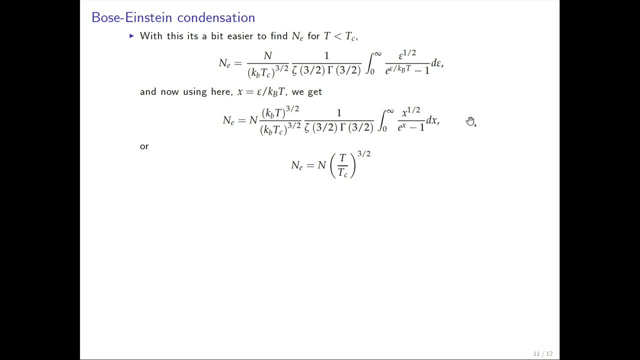 and in the end we get a pretty simple expression. this way, I mean, like I said, you could do it the long way. you just get the same thing. you just have to do a bit more algebra and what we see is a simple kind of result that the number in the excited state below 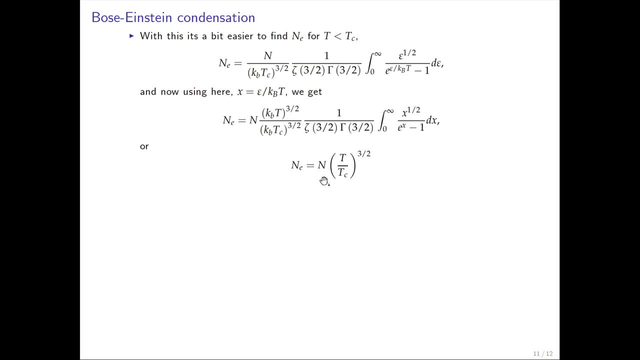 Tc, so we're at T below Tc. is the total number times T over Tc to the 3 halves power. ok, that's from these terms, because all this cancels out in the end, ok, and and then. so if we divide this by N, 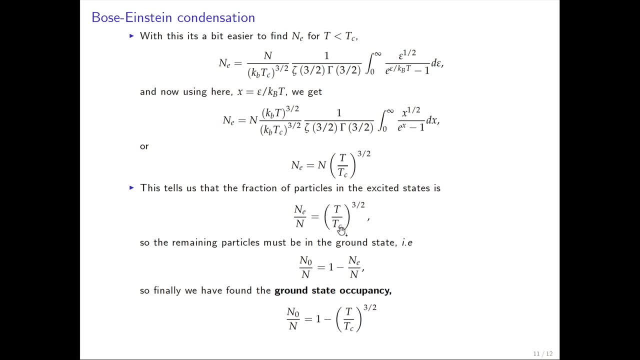 that's the fraction of particles in the excited states. it's just T over Tc to the 3 halves, and so the remaining fraction must be in the ground state. that is the fraction. the fraction of particles N0 over N in the ground state must be 1 minus. 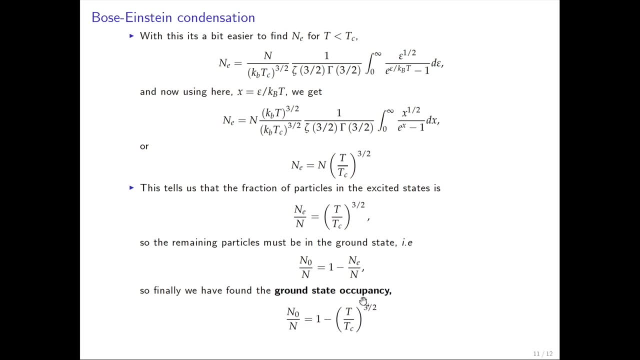 this fraction. so we can write it out as: N0 over N equals 1 minus T over Tc to the 3 halves power. so this tells us quantitatively what we had argued was happening, that below Tc we get a large number of particles. 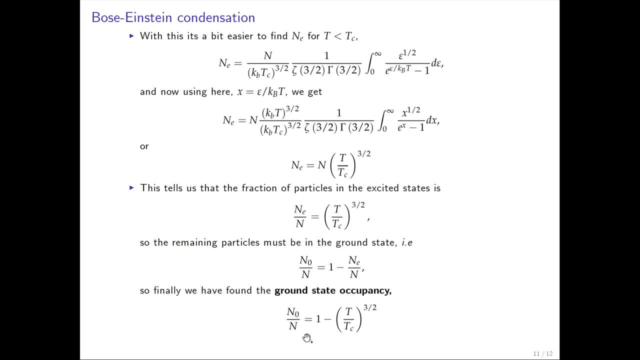 in the ground state, the fractional occupancy gets very, very large, which means we have a large number in the ground state until we get to T equals 0, when all the particles are in the ground state. but this actually tells us the form of that, and so that's. 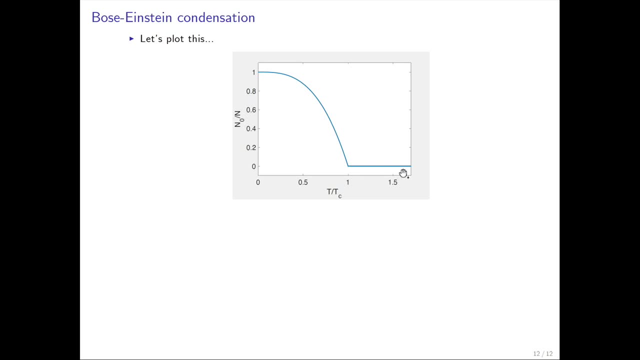 so we plot that. of course it looks like this. so this number in the ground state is infinitesimally small above here and in the thermodynamic limit, in the limit where N goes to infinity, it really is 0 up here and it goes like this below. 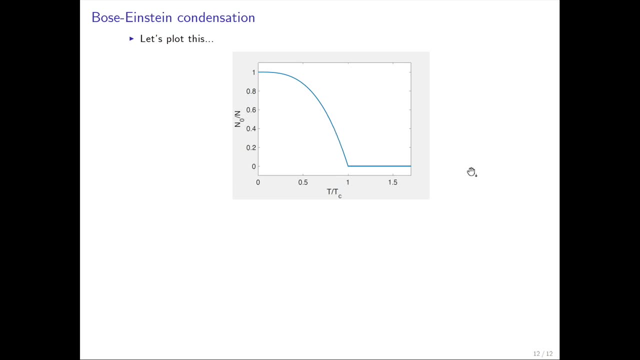 this is the power law. we predicted: T over Tc squared, or Tc to the 3 halves. ok. so for T greater than Tc, the number of particles in this ground state is actually negligible, and in fact, for N, the total number of particles going to infinity. 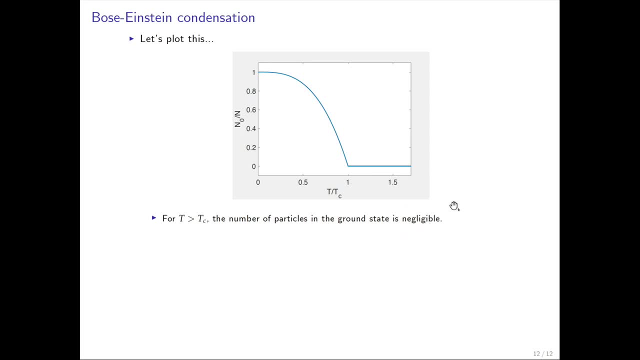 it really does go to 0 there, and this becomes very sharp, and so, below Tc, the number of ground states increases rapidly, and this is a phenomenon of what's called Bose-Yanssen condensation. ok, now, this growth that starts out from 0 essentially tells us that. 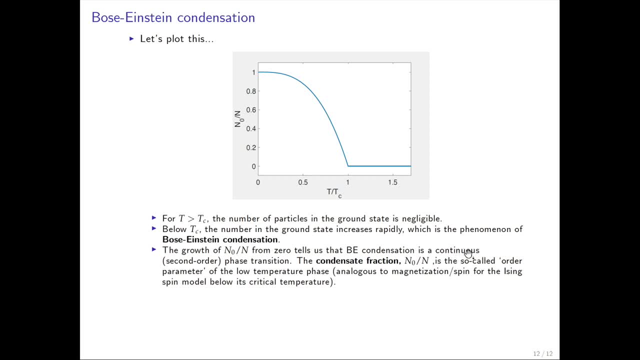 the Bose-Yanssen condensation is a phase transition and, moreover, it's a continuous phase transition, also known as a second order phase transition. in continuous or second order phase transitions, you have what's called the order parameter, which grows from 0 and so this constant fraction. 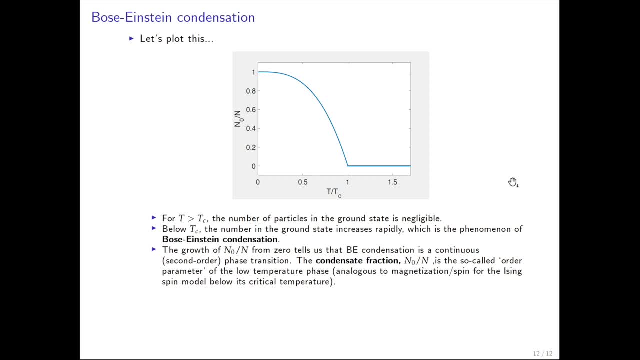 for this type of condensation is the order parameter. another example of order parameter, by the way, is the sort of magnetization, magnetization per spin. technically so this is like fraction and this is sort of like magnetization per spin for the icing model. spin model of one second order phase transitions.